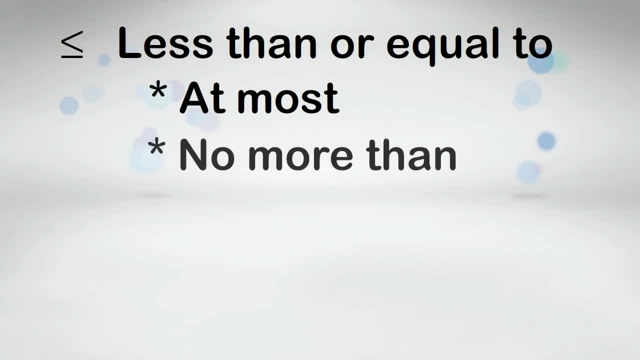 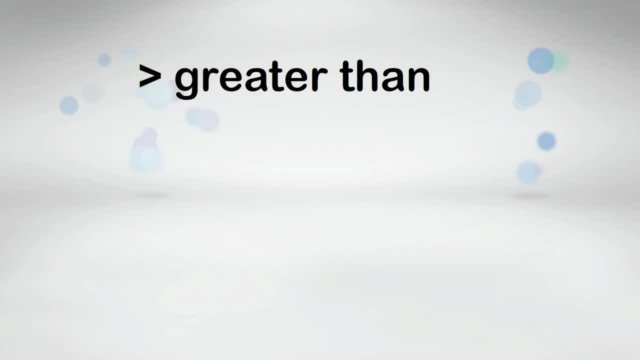 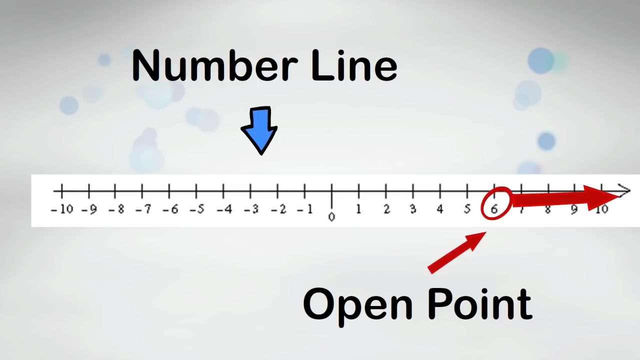 It is also expressed as: at most no more than a maximum of or any more than Up next is greater than also called more than. Finally, less than also can be called fewer than On a number line. if you have an open point, it means the number is not included in the solution. For example, x is greater. 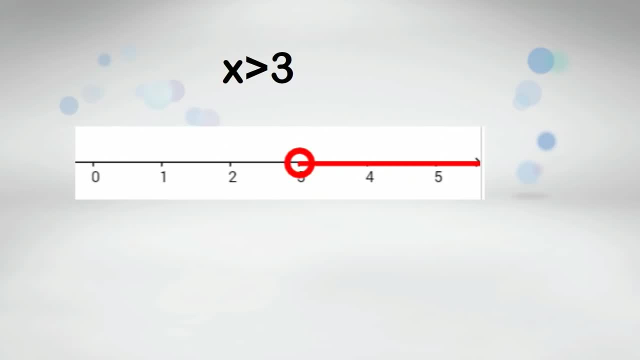 than 3.. Notice that you use an open point because 3 is not included. x is less than 6.. Again, an open point is used. The next symbol is less than or equal to. It also may be expressed as less than or equal. 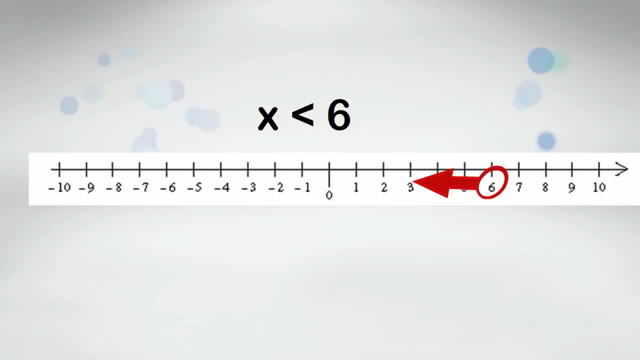 to. The following symbols are used to express inequalities: The following symbols are used to express inequalities: The following symbols are used to express inequalities: The following symbol is used to express inequalities: The following symbols are used to express inequalities: In this example, x is looking for the equal or equal cos. 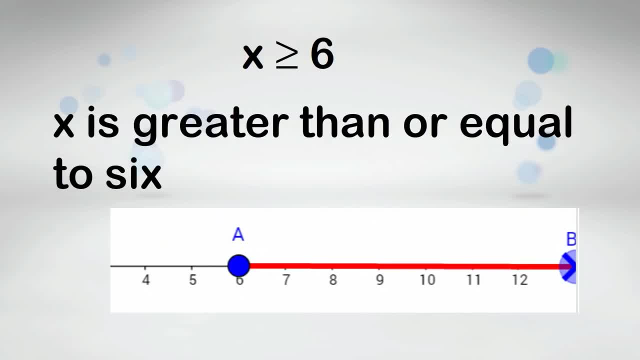 x is looking for the equal or equal sin. Observe in the following form: until you are completely confident, Scholar says that the number is included in the solution. A closed point means that they large number is included in the solution. X is greater than or equal to 3.. A closed point is included because 3 is included. X is greater than 6.. 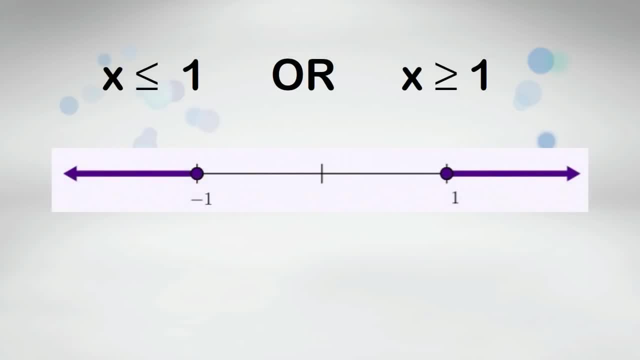 The graph will point in two different directions. If the variable is in the middle of two inequalities, the graph will be used between the two points. For example, 4 is less than x, which is less than 9.. Let's look at some more examples. 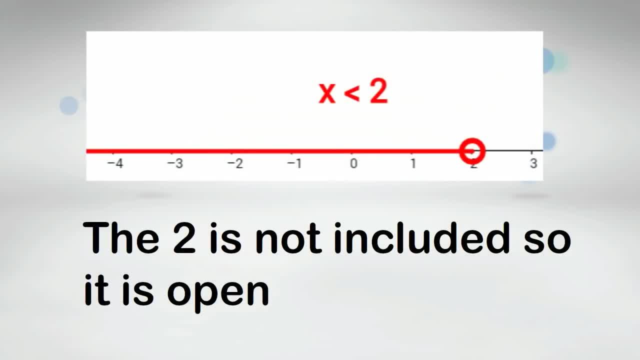 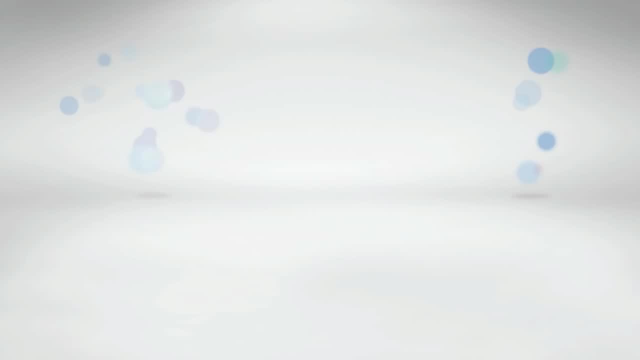 X is less than 2.. 4 less than will not be included, so it will be open and the 2 will not be included. X is greater than or equal to 10.. In order to graph this inequality, it will be closed and the 10 is included. 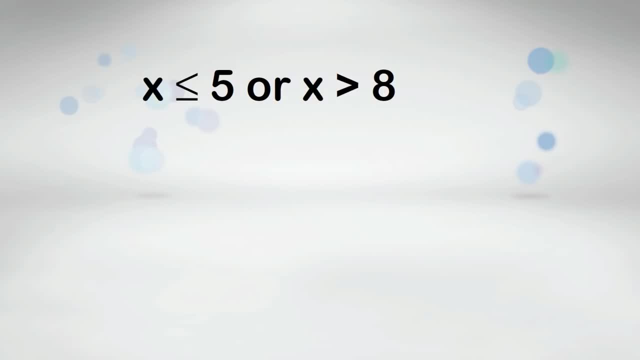 X is less than or equal to 5, or x is greater than 8.. This inequality will point in two different directions, because it uses: OR 3 is less than or equal to 5.. 3 is less than or equal to 5..